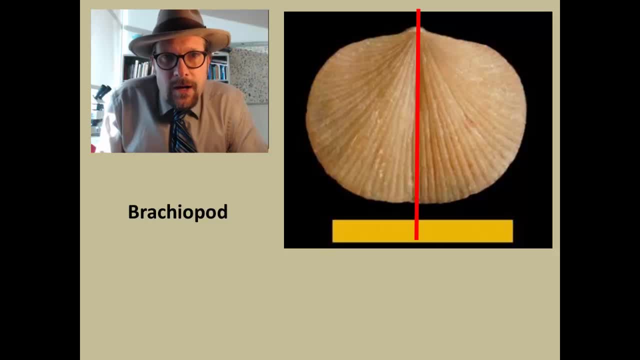 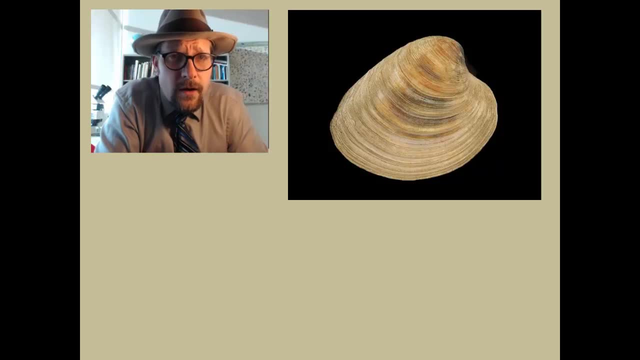 It does. So we know that this is a brachiopod. Now take a look at this shell. What do you think? Do you think this is a brachiopod, or do you think it is a bivalve? Well, it is a little hard to draw a straight line through this, to split it evenly, so there. 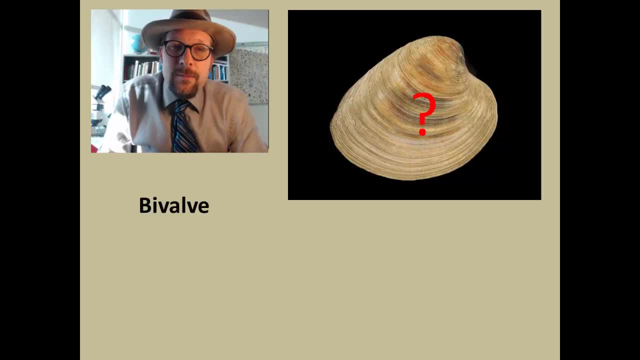 is no real symmetry. We know that this is actually a bivalve, and so that is the major way of telling the difference between brachiopods and bivalves such as clams and oysters. This symmetry has to do with the way in which the shell grows, and we will look at how brachiopods 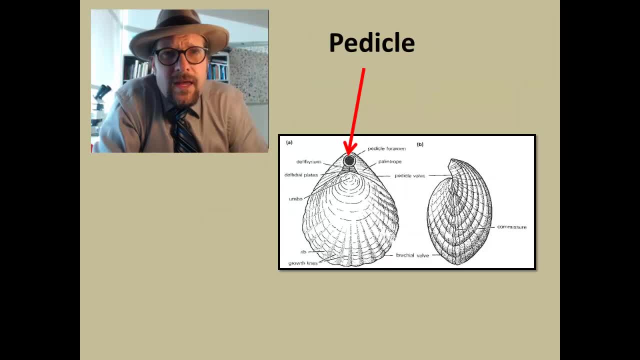 grow later on in this lecture. Let's now talk about the anatomical terms for brachiopods. The anatomical term for brachiopods is brachiopods. The anatomical term for brachiopods is brachiopods. The anatomical term for brachiopods is the. 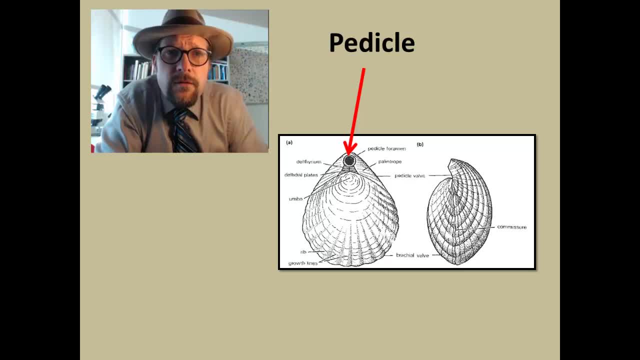 anatomy of brachiopods. The anatomical term for brachiopods is the anatomy of brachiopods. To describe the anatomy of brachiopods, the first feature is the pedicle. This is the fleshy stalk that attaches the brachiopod to the seafloor. Not all brachiopods have. 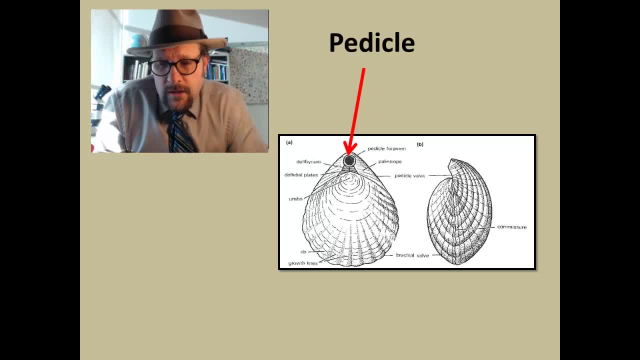 a pedicle. Some are free-laying and some have a broad hinge line instead. The umbo is the raised protuberance on the shell, which is the initial growth stage of the shell. The commissure is that line where the two halves of the shell meet. 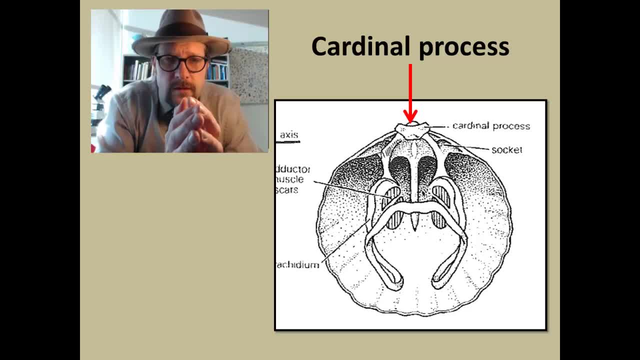 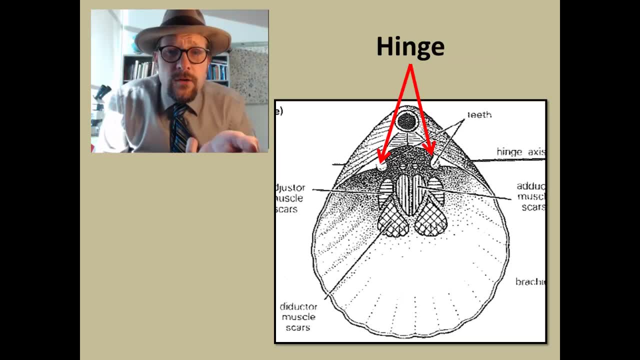 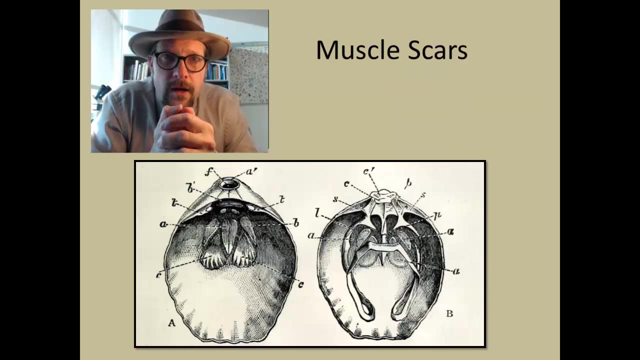 These shells are actually attached via a cardinal process. The cardinal process is named because it kind of resembles a heart. This process fits into two hinges that are paired and have teeth that connect in with the cardinal process. Brachiopods have three sets of muscles and these muscles work together to provide movement. 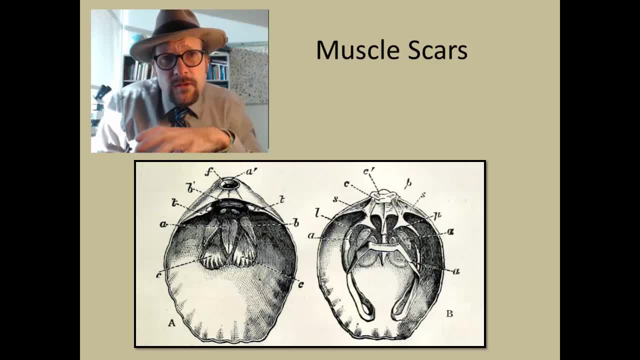 of the shell. These muscles can be seen in muscle scars in both of the shells. The first one we will look at is the adjuster muscle. This is a muscle group that move the pedicle stocks. They run from the pedicle side of the shell up through the pedicle and attach to the stock. 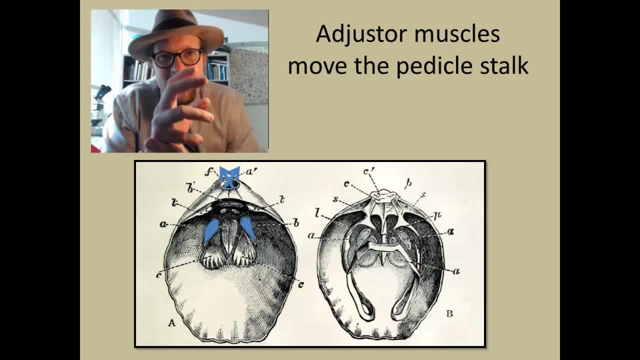 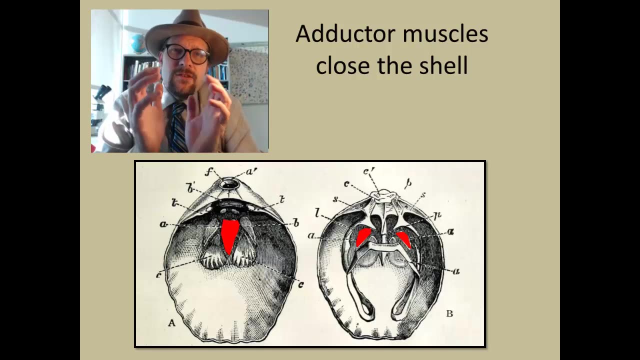 The adjuster is referring to the fact that these muscles adjust the position of the brachiopod by flexing that muscle. The next muscle scar is the adductor muscles. These are found on both halves of the shell. The adductor muscles constrict and pull the two halves of the shell together. 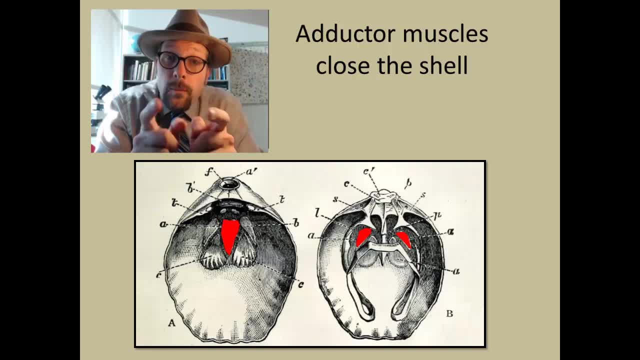 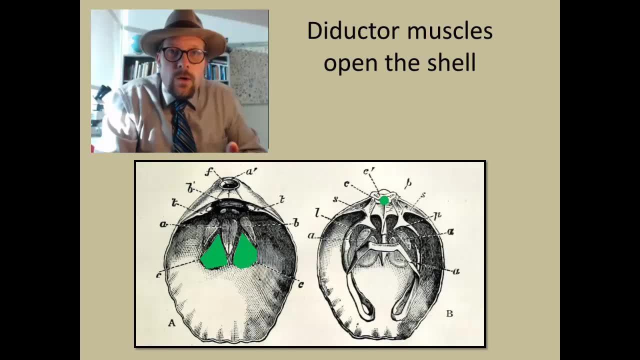 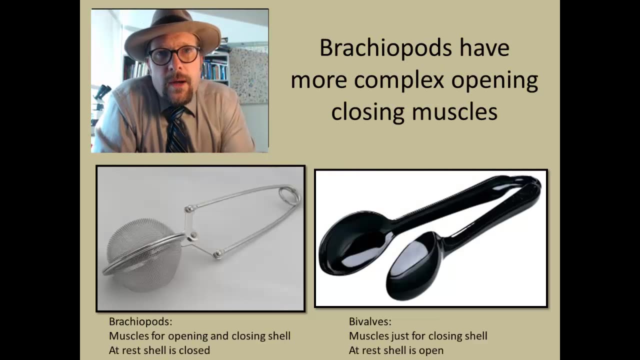 Hence they are called adductor muscles, since they add or bring together the two shells. The final set of muscles are the diaductor muscles, which connect one shell with the cardinal process. When it flexes, it closes the shell. What is remarkable about brachiopods is that with these three sets of muscles they can 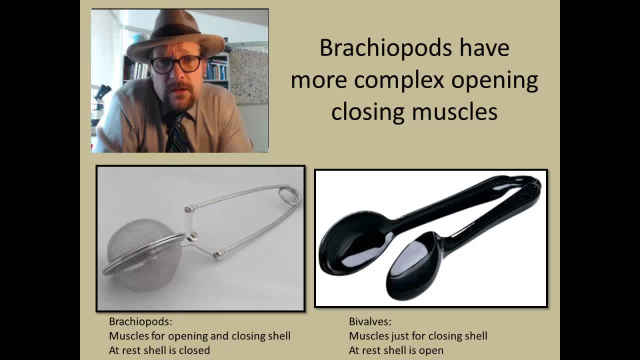 both open and close. They can close their shells by constricting their muscles. This is very different from what is found in clams and other bivalves, which have only one set of muscles and when relaxed they open. Hence, if you do a clam bake, the clams will open when the clam is cooked and as these 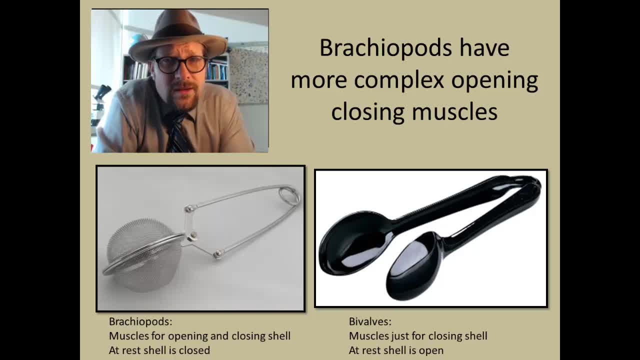 muscles relax In brachiopods, the resting condition is a closed shell. This means that muscles are constricted to open the shell. So if you were to do a brachiopod bake, the brachiopods would likely stay closed until. 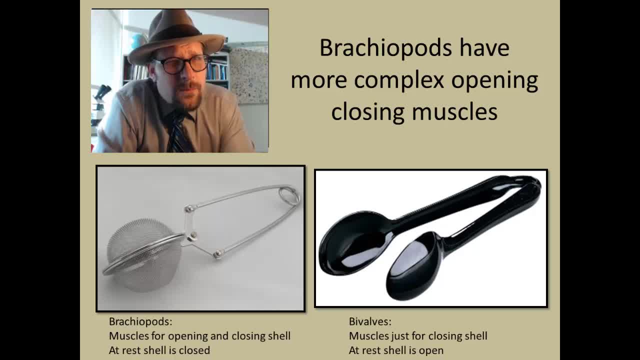 you force them open. Few people eat brachiopods, and when they do, they eat the fleshy stalks instead. These different styles of tongs nicely illustrate the functional difference between the two groups. 1. Brachiopods are for opening and closing the shell, whereas bivalves only have a muscle. 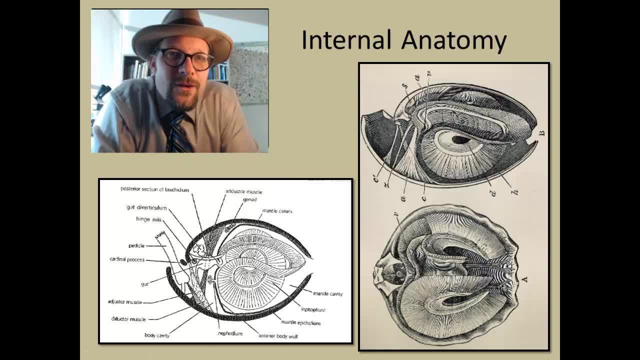 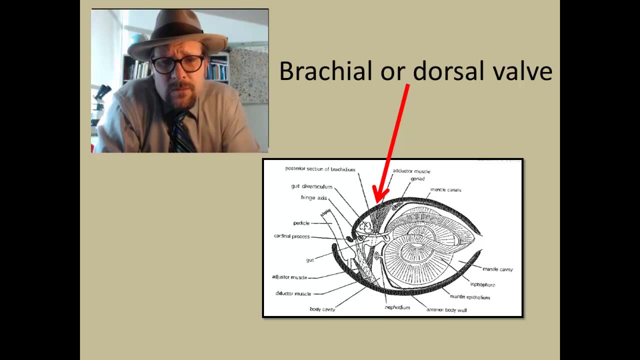 that contracts and closes the shell. Now let's look at the rest of the internal anatomy of brachiopods. To reference the position of an animal without a head or tail, we have to use some anatomical names. The smaller shell is the brachial or dorsal valve, the lower one that contains the pedicle. 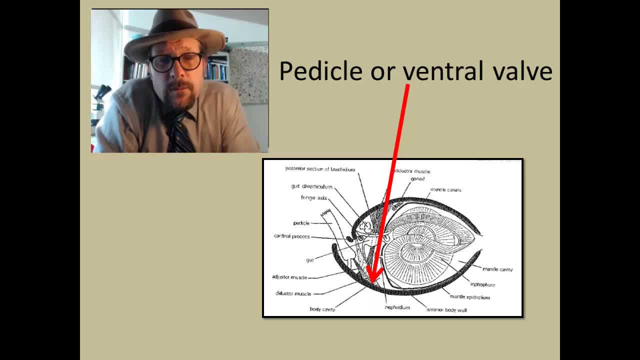 and the ventral valve, the larger of the two shells. 2. The posterior end is the end with the stock. 3. The anterior end is the end with the commissure. Inside the brachiopod is a large lofophore. 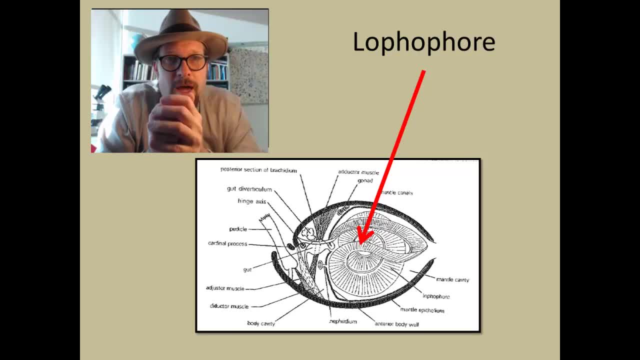 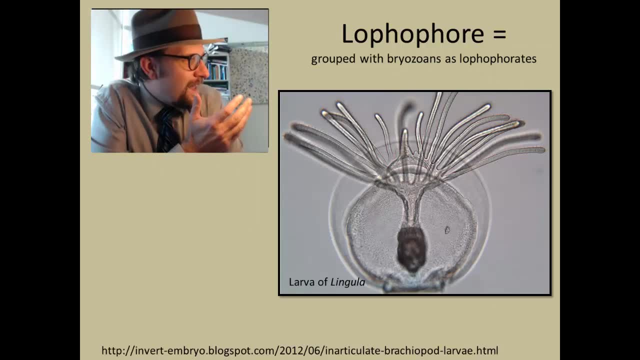 This lofophore opens up and is used to filter food out of the water. The lofophore is similar to what we saw in bryozoans. in fact, here is a larval brachiopod. Look at this larval brachiopod and realize how close it resembles the zooid bryozoans. 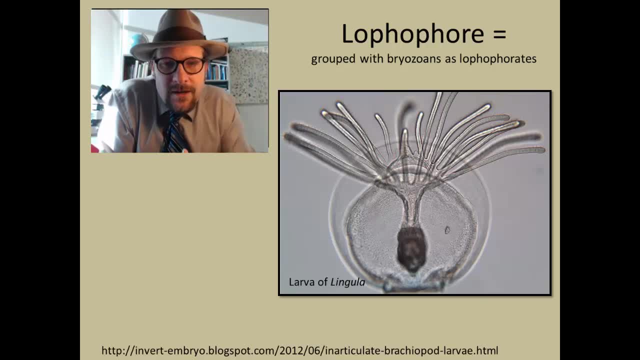 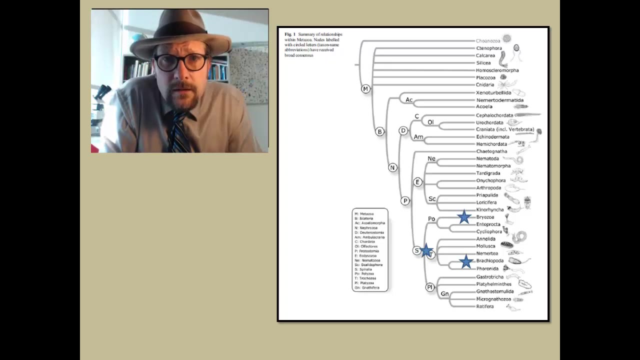 with its large lofophore and its small paired calcite shells. Interestingly, brachiopods have a fossil record that predates the bryozoans and are known from the Cambrian. Phylogenetically, brachiopods and bryozoans are closely related and, although more recent, 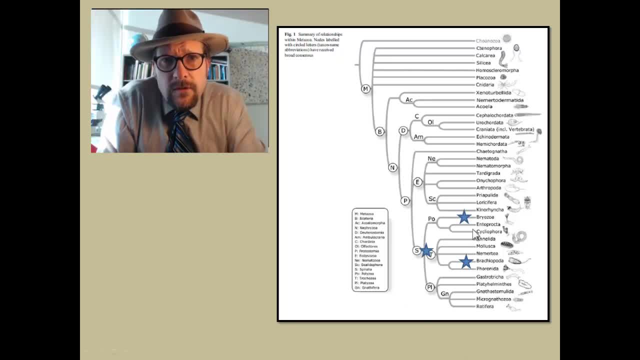 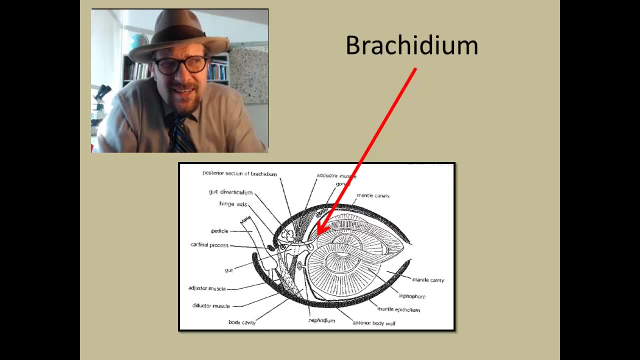 molecular phylogenies have separated them out a little bit, mostly by inserting some of these groups that do not fossilize very well. brachiopods and bryozoans are in the same group. The lofophore is supported by a calcite brachiodome, which is like an internal skeletal support. 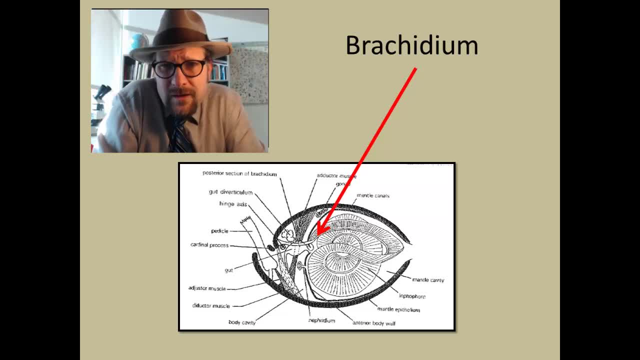 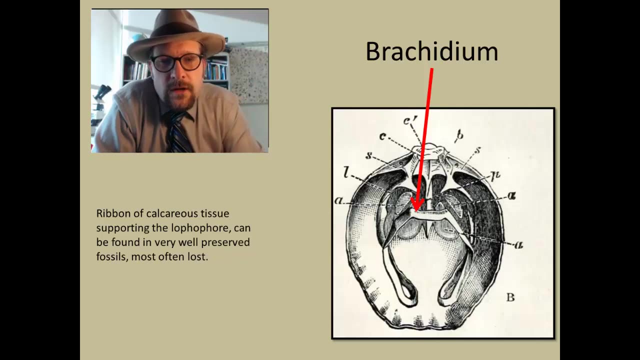 for the lofophore. The brachiodome rarely fossilizes, but it can be found inside some fossil shells, although most often it is not preserved. because of its delicate nature In shells it tends to be a loop-like feature that is often preserved in modern brachiopods. 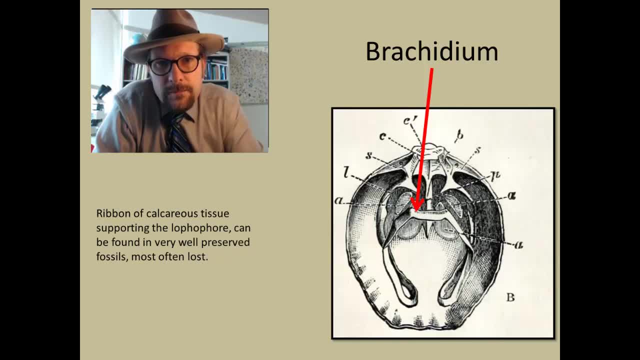 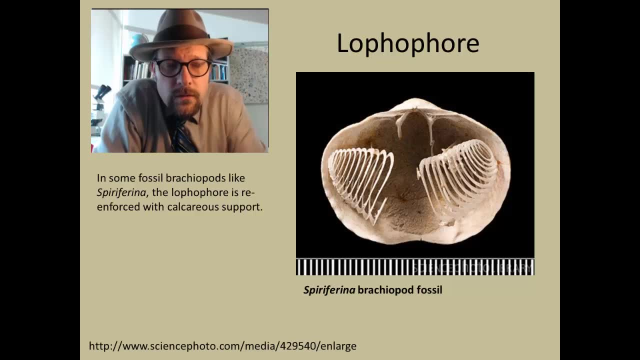 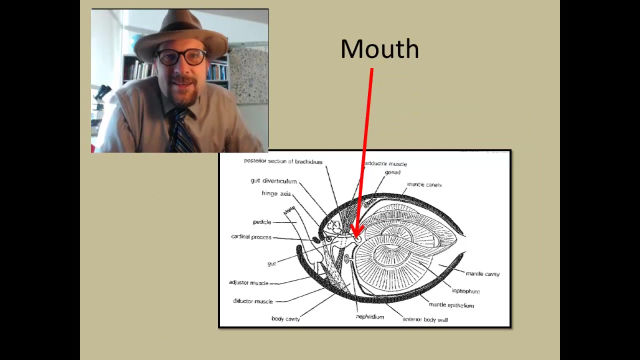 In some brachiopods, like Spinarifia, the lofophore is reinforced with a calcareous support which more often is preserved, especially in delicate specimens prepared using acid. The lofophore functions to get the food into the mouth and is analogous to the hands of 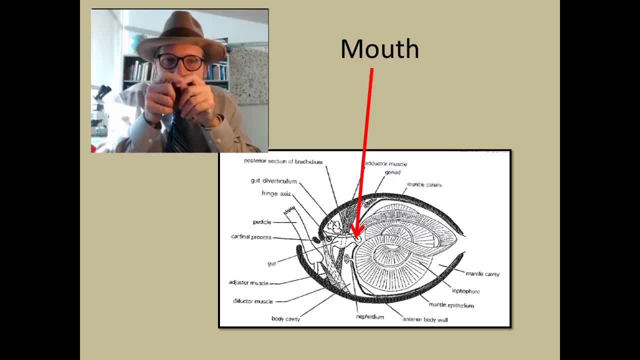 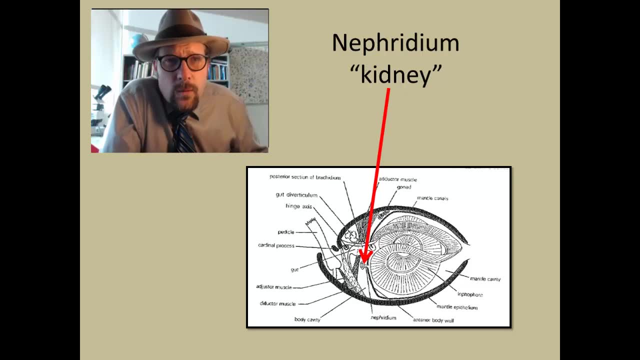 the brachiopod. Arrrrgh, Arrrrgh, Arrrrgh, Arrrrgh, Arrrrgh, Arrrrgh, Arrrrgh. Brachiopods also have an organ called an ephedrine, or kidney, that helps regulate water and waste. 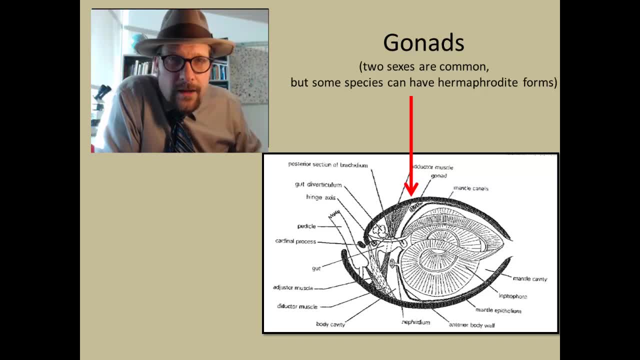 The final organs in the interior of the shell are the gonads. these are the gamete cells that produce the sperm and eggs. There are boy and girl brachiopods, but some brachiopods are also hermaphroditic and produce. 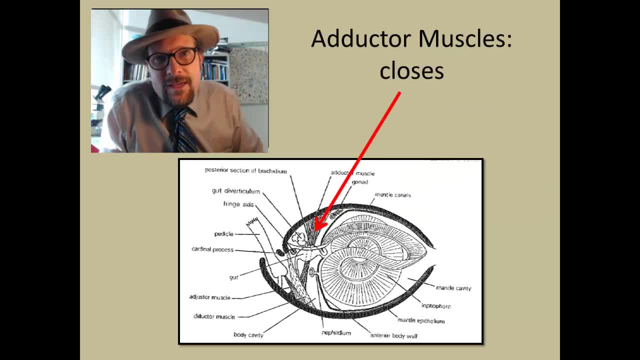 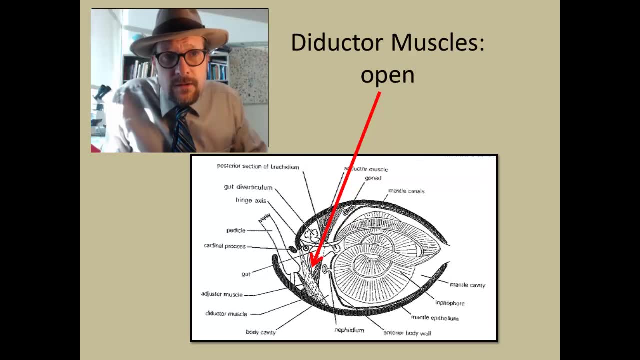 both sperm and eggs. Lets go over the muscles again, since they are part of the interior anatomy. The adductor muscles close the shell running between the two shells. The diductor muscles open the shells running from the ventral part of the shell up to the 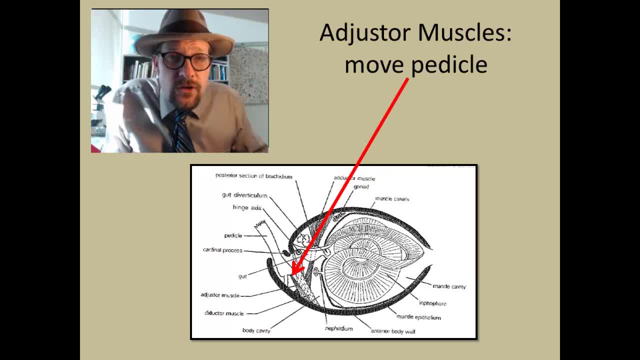 cardinal process. The adjustor muscle moves the pedicle, so it runs from the ventral shell up to the pedicle or the stock to help move and adjust its position. One other term that is unique to brachiopods is the adductor muscle. 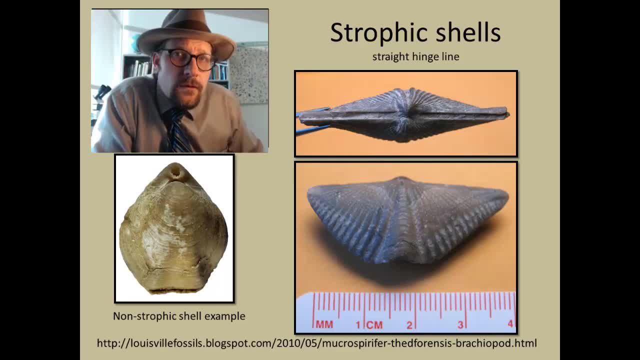 It is the adductor muscle that moves the pedicle. It is the adductor muscle that moves the pedicle. The other term that is unique to brachiopods is the strorophic. This refers to the hinge being in a straight line. 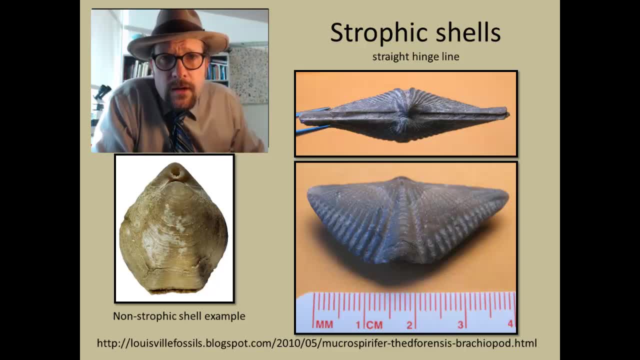 Strorophic brachiopods are common in the late Paleozoic in having a straight hinge line. The one below is a non strophic shell as an example of how different these hinge lines can be. Another term is a zigzag commissure. 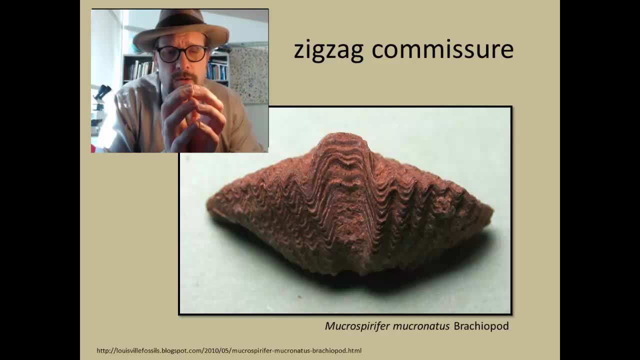 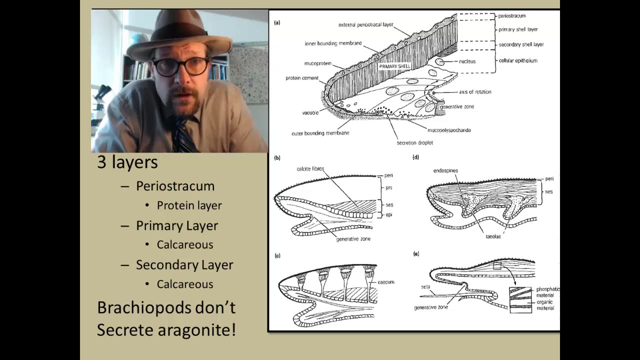 With this, there are two sides of the shell are growing and they grow in its. Now let's take a look at how brachiopods grow their shells. There are three layers associated with shell growth. The outer layer, the first layer to be secreted by the cells is the perioscium, which is 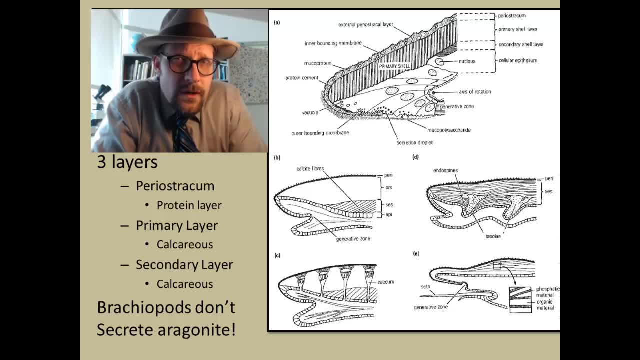 composed of protein. Since it is organic carbon, it tends not to be preserved in the fossil record. The next layer is the primary layer, which is composed of calcite. This is laid down on the outer margin of the shell. As the shell grows, a second layer of calcite is laid down. 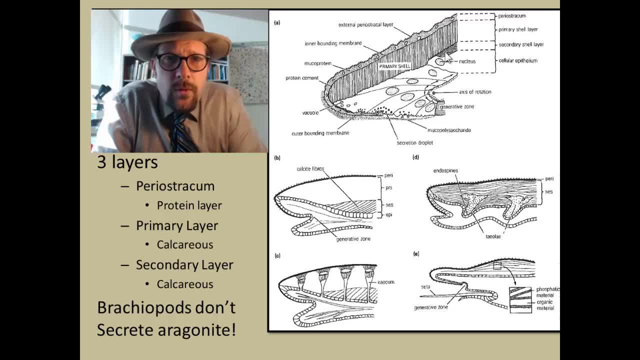 This thickens the shell further. An important point is that brachiopods don't secrete aragonite. Aragonite is found in bivalves and it is the mineral that forms pearls, So brachiopods don't form pearls. 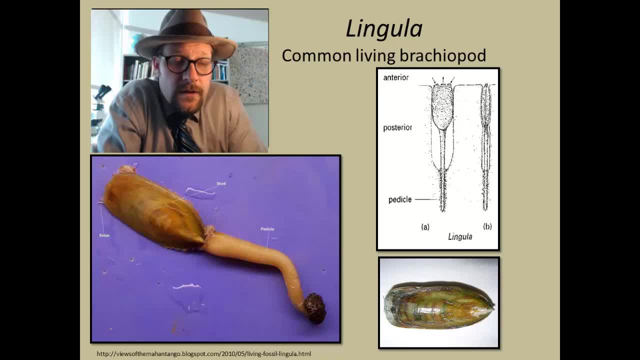 The most common living brachiopod is Linguia. Linguia is found in abundance in offshore cooler waters. It tends to favor deeper waters. Linguia is a living fossil because it has an extensive fossil record that extends all the way back to the Paleozoic. 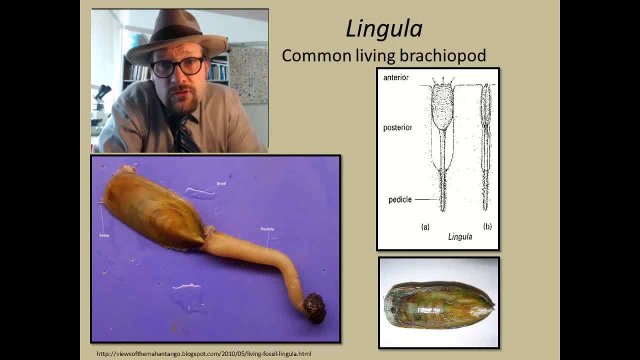 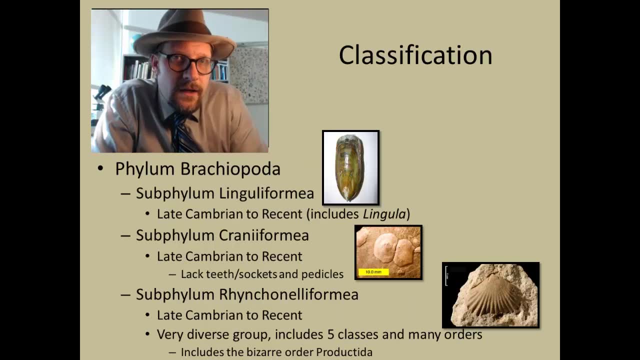 It lives in the mud and uses its fleshy stalk to retract into burrows and into the mud It is commonly found as a fossil. Now let's look at the classification of brachiopods and recognize the three major groups. The first group is the subphylum. 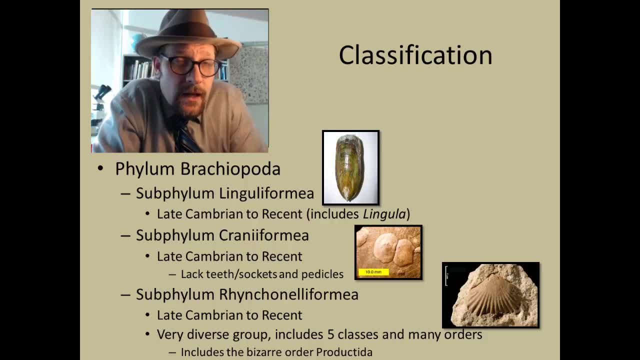 Subphylum is the subphylum. The subphylum is known as Linguia forma, known from the Late Cambrian to the Recent. This includes Linguia. The second group is the subphylum Creniforma, from the Late Cambrian to Recent. 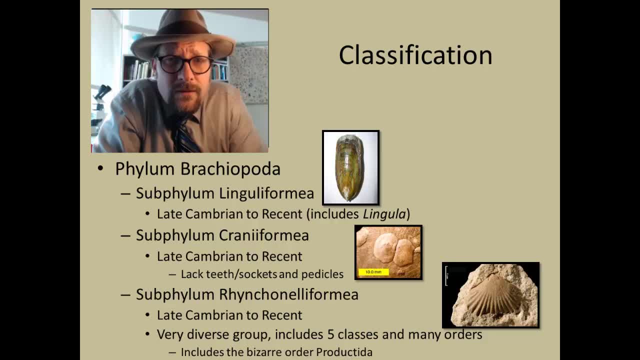 These are unusual forms in that they lack teeth and sockets and lack pedicles. They are also often found open And the most diverse group is the subphylum Rhenichnella forma, from the Late Cambrian to Recent. It is a very diverse group. 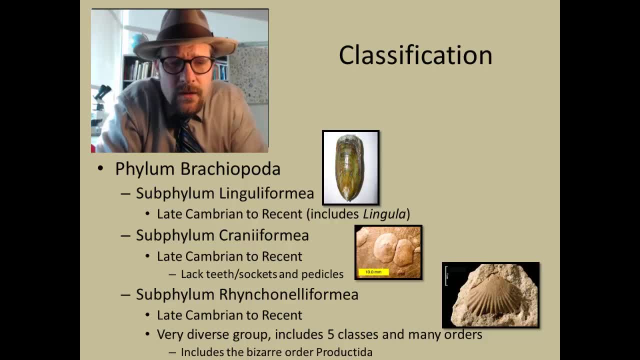 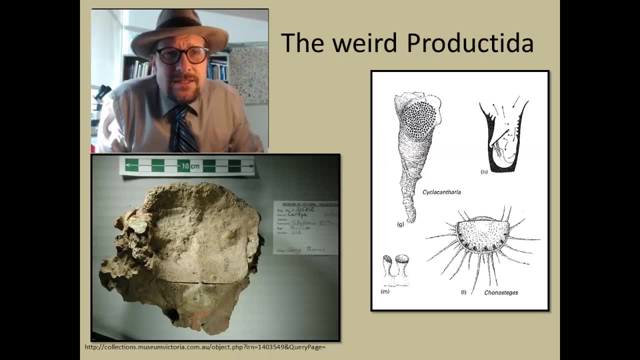 There are five different classes. The most diverse group is the subphylum Rhenichnella forma, from the Late Cambrian to Recent. I will just highlight one in group and that is the Bizarre Order Producta. Producta is a weird brachiopod. it actually forms reefs and it has a shell that opens. 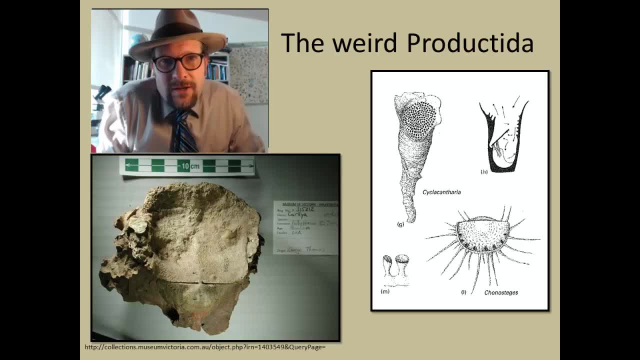 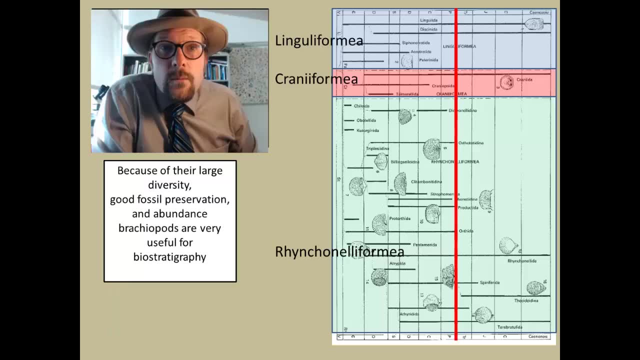 and closes, but it grows into these weird tube-like shells, very different ventral and dorsal shell anatomy, known from the Lower Devonian to the Upper Permian. Because of their large diversity and good fossil preservation and abundance of brachiopods. 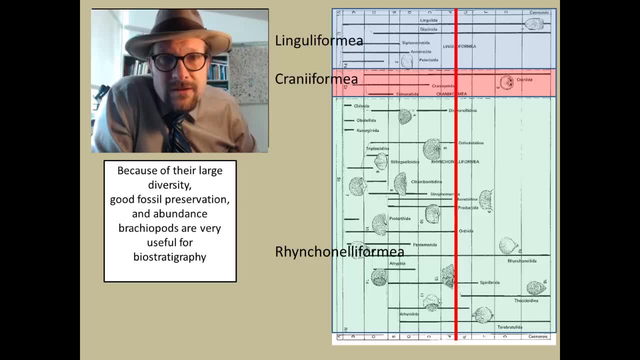 they are very useful for biostratigraphy. All three groups extend to the recent. however, during the late Paleozoic brachiopods were much more diverse. The end Permian extinction, shown here in red, really pruned back the brachiopod tree. 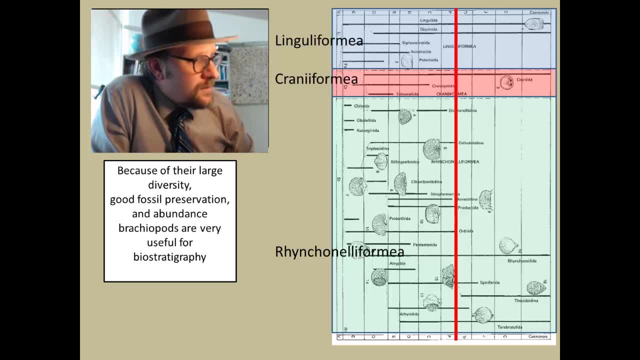 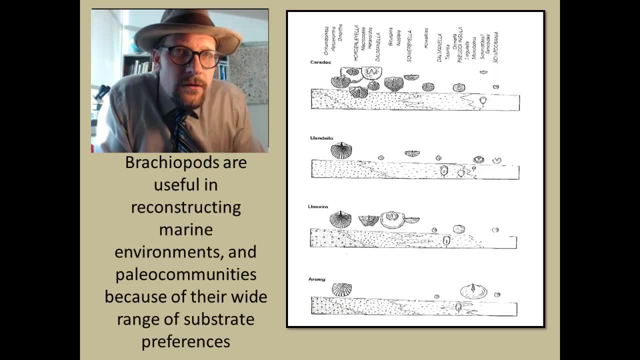 with a number of branches surviving to today, Because they are so common. they are very rare And they are really great index fossils for the Paleozoic era. Brachiopods are useful for reconstructing marine environments and paleo communities because of their wide range of substrate preferences. 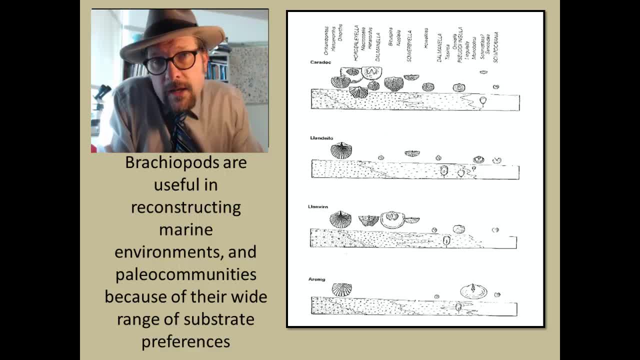 Diversity, patterns and ecological recoveries can be studied using brachiopods, because their habitats and niches can be resolved in the fossil record. Hence the study of brachiopods is really important in paleontology and geology in general, because of their common occurrence and their usefulness in biostratigraphy, aging rocks and reconstructing.